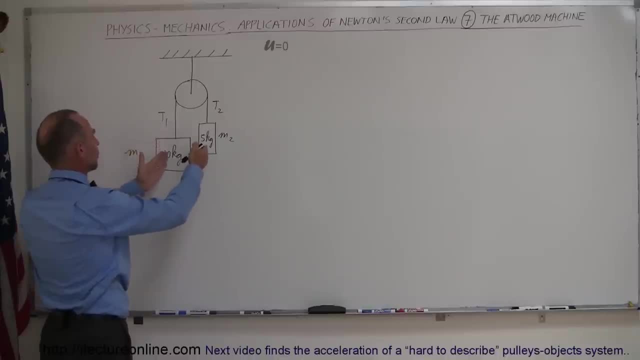 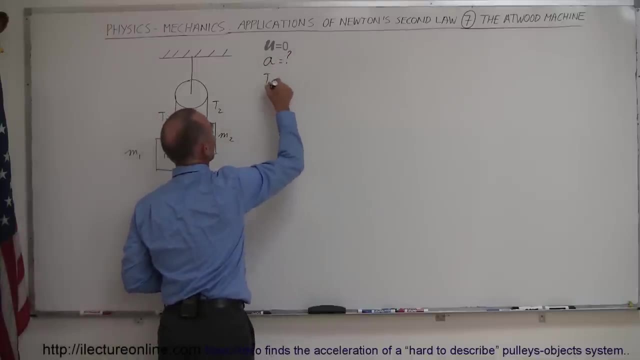 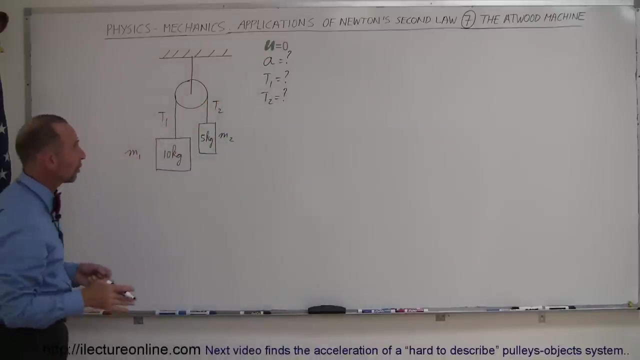 you can see that there's going to be an acceleration. the heavy mass is going to be accelerating downward, the lighter mass is going to be accelerating upward. What is the acceleration of the system and what is the tension on the strings? And, of course again, if the mass, if the pulley has no mass and no friction, you 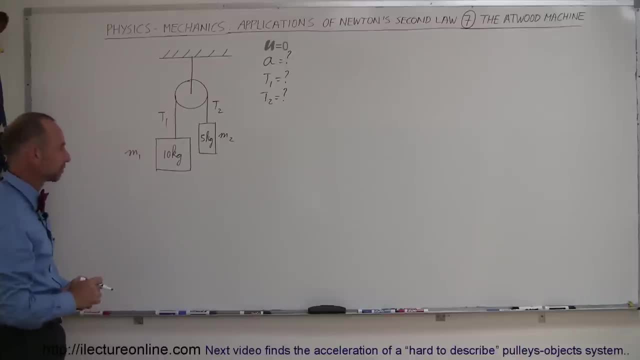 would expect T1 and T2 to be the same, which in this case it is. Alright, let's draw all the forces acting on the system. So again, I'm going to find the acceleration by looking at this as a singular system. right here We have M1G. 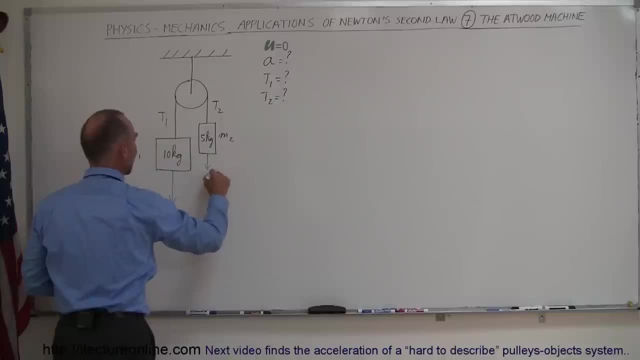 pulling down in this direction, and we have M2G pulling down in this direction Now, which is bigger. M1G is bigger and since everything is connected, you would expect the whole system to be accelerating this way. So I'm going to call acceleration in this direction as 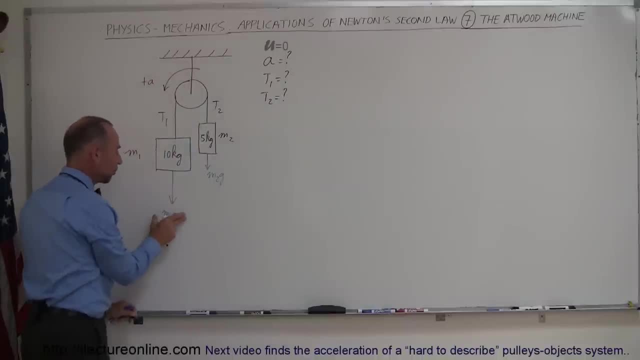 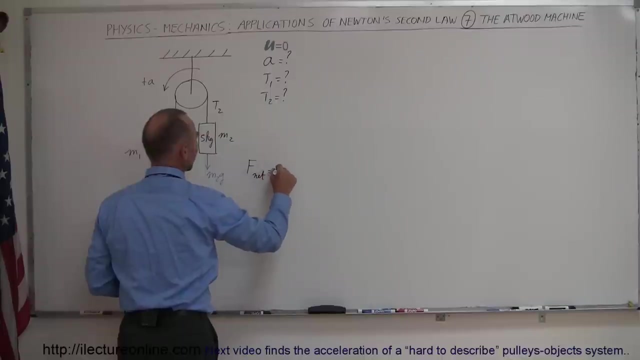 the positive direction And then this force would be aiding the acceleration. same direction of acceleration. This force would be opposing the acceleration because it's in the opposite direction of acceleration And, of course, using Newton's second law, we can write: F: net equals mass, total times acceleration. 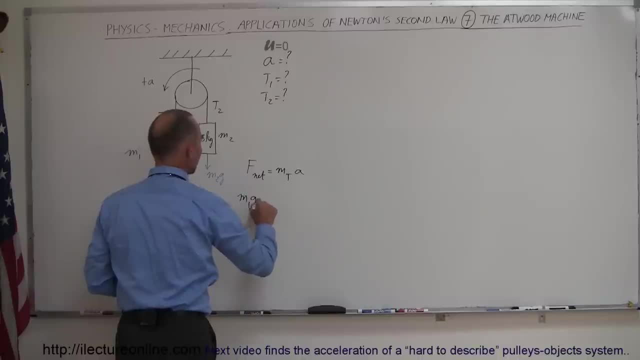 The net force then of course would be M1G, which aids the acceleration, minus M2G, which opposes the acceleration, equals the total mass, M1 plus M2 times the acceleration. And of course, at this point, if we divide both sides by M1 plus M2, we have the equation: 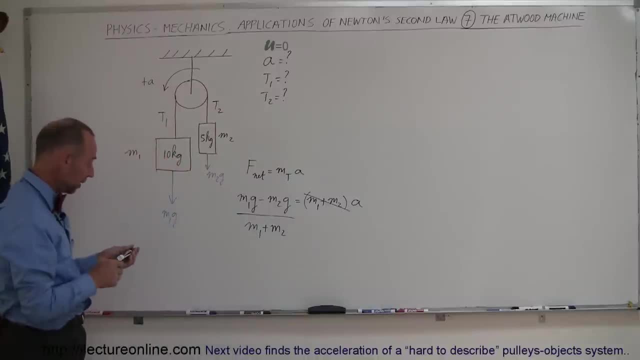 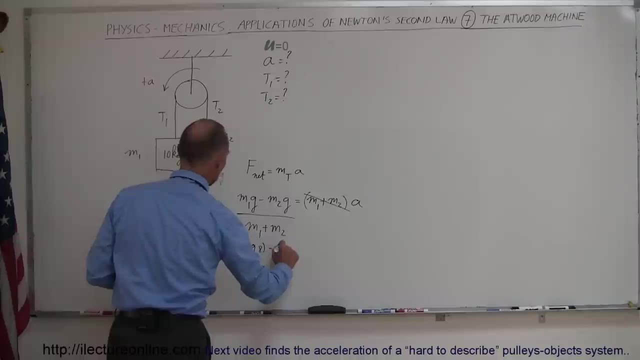 for the acceleration of the Atwood machine. Now let's plug in the numbers. So M1 is 10G- 9.8.. Minus M2, which is 5, times G, 9.8, all divided by M1 plus M2,, which is 10 plus 5.. And of 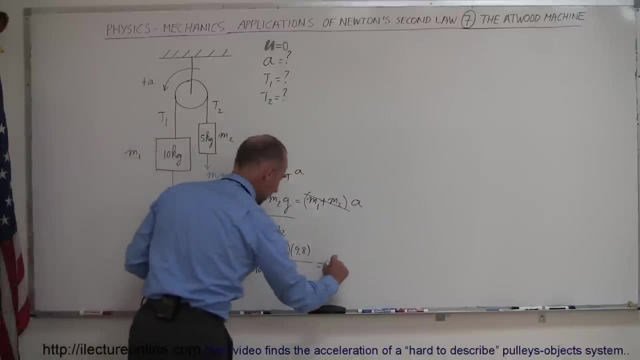 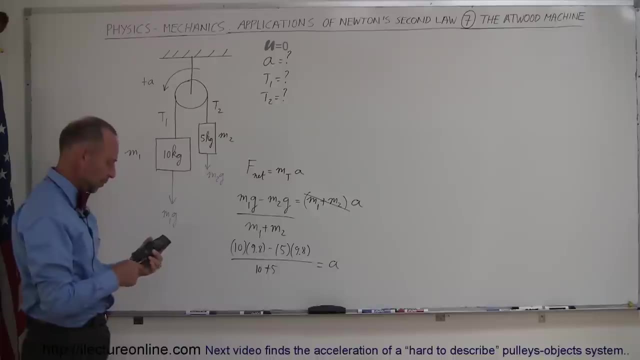 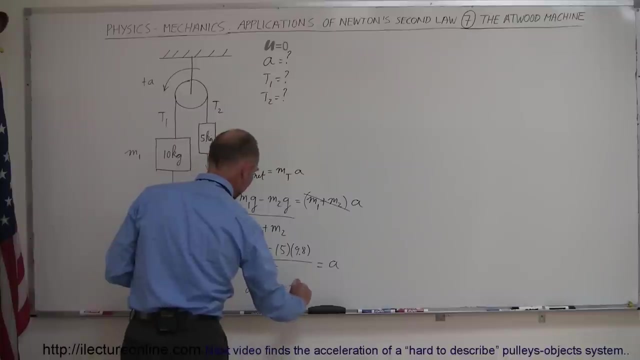 course, the units are going to be meters per second squared. This is the acceleration. And let's see here: We have 49 divided by 15, which would be 3.27 meters per second squared. So acceleration equals 3.27 meters per second squared. 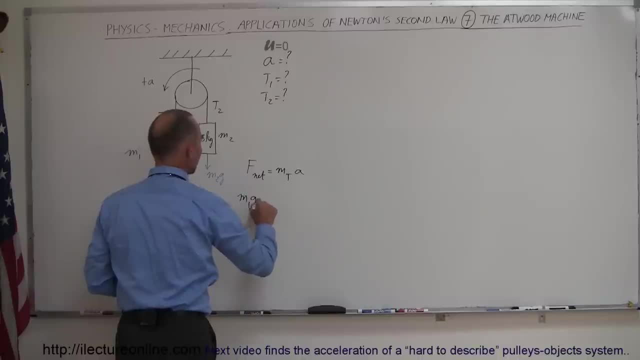 The net force then of course would be M1G, which aids the acceleration, minus M2G, which opposes the acceleration, equals the total mass, M1 plus M2 times the acceleration. And of course, at this point, if we divide both sides by M1 plus M2, we have the equation: 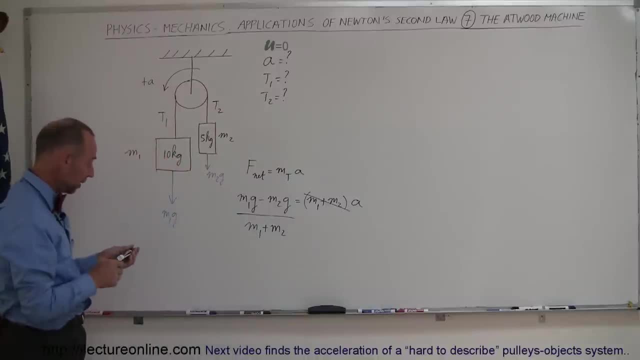 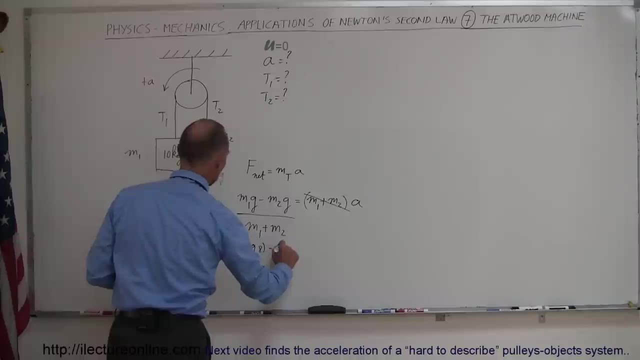 for the acceleration of the Atwood machine. Now let's plug in the numbers. So M1 is 10G- 9.8.. Minus M2, which is 5, times G, 9.8, all divided by M1 plus M2,, which is 10 plus 5.. And of 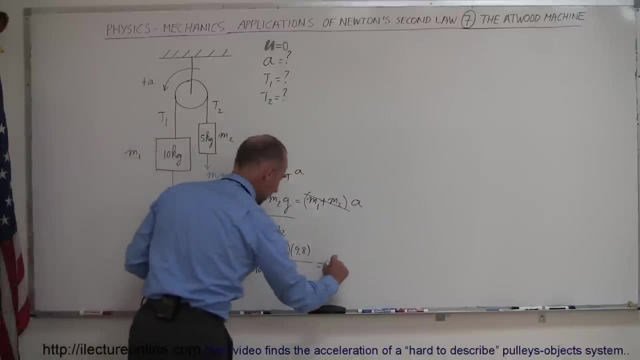 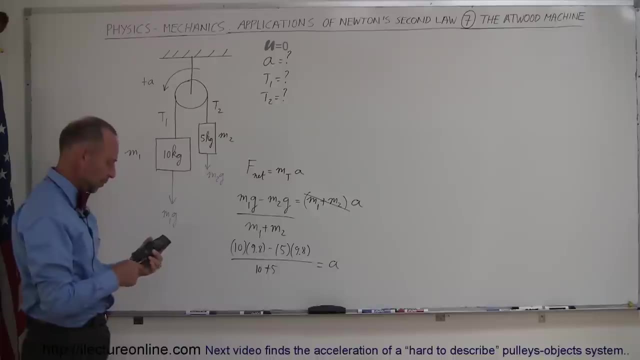 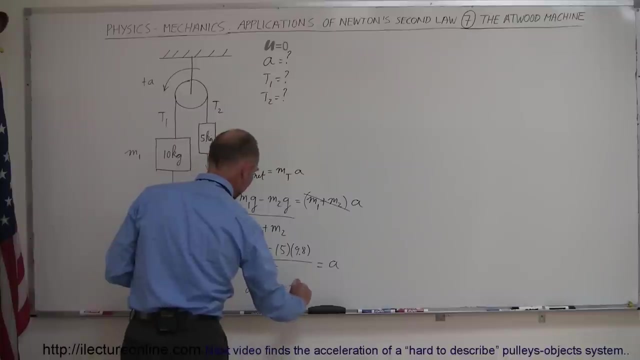 course, the units are going to be meters per second squared. This is the acceleration. And let's see here: We have 49 divided by 15, which would be 3.27 meters per second squared. So acceleration equals 3.27 meters per second squared. 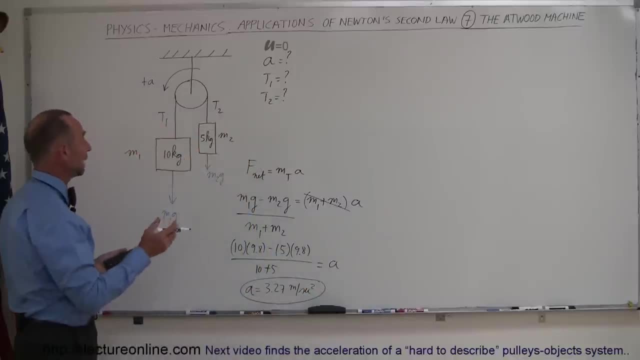 All right Now to show, for one, that tension one will equal tension two, and to show how easy it is to apply this concept of how to calculate the tension of the string on both sides of this pulley. let's start with tension one first, And here we can see that, since 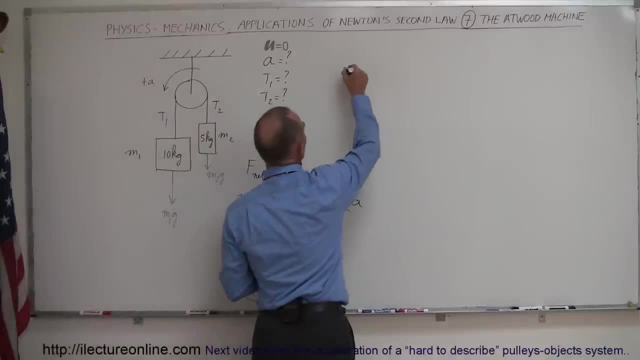 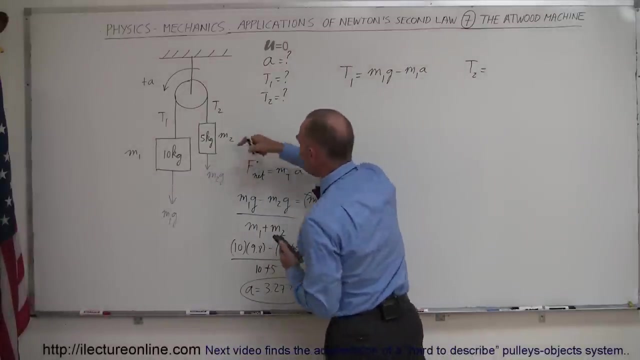 mass one is being accelerated downward, we can say that tension one is equal to the weight of that object, M1G minus M1A, because it's accelerating downward. To find tension two, we can say that it's equal to the weight of this object, which is M2G, But since M2 is being 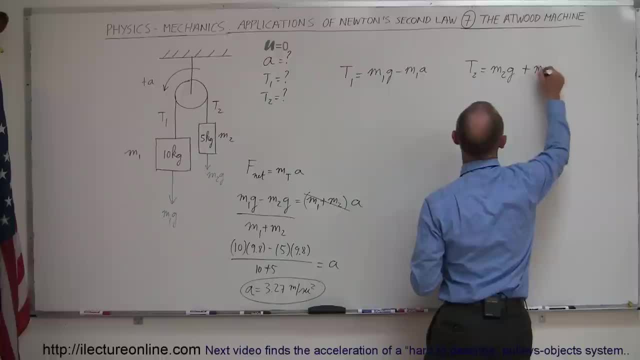 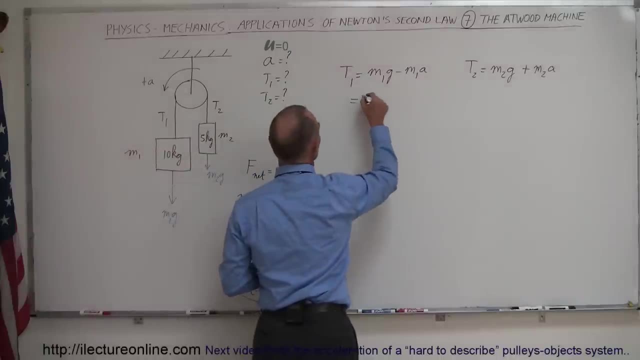 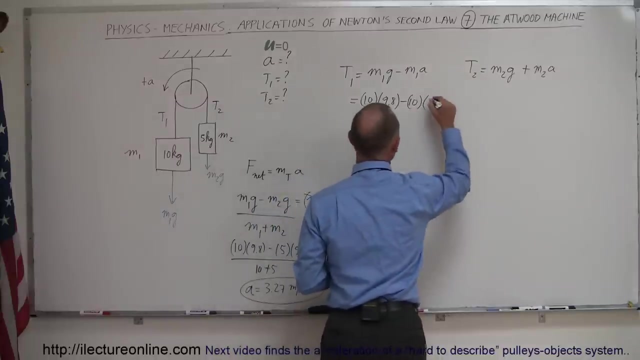 accelerated upward. we have to write plus M2A, And those should be equal to each other. So let's plug in the numbers and find out. So this is equal to 10 times 9.8 minus 10 times 3.27..